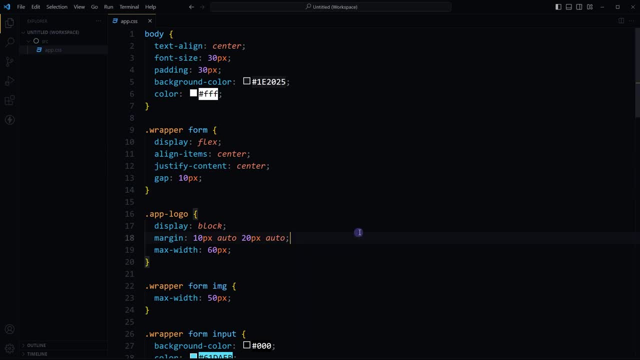 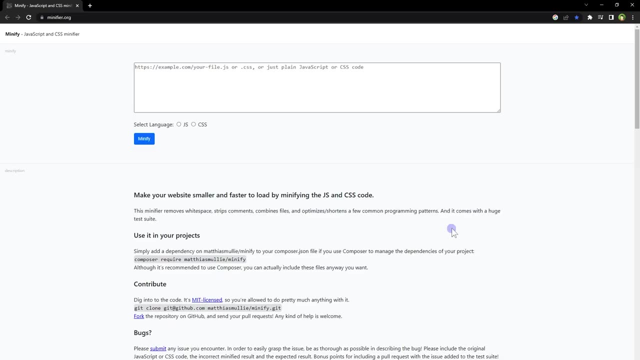 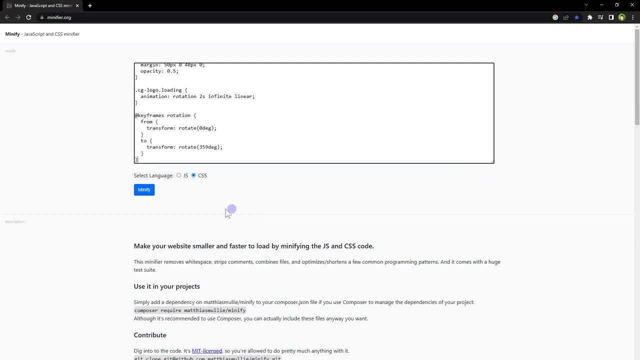 topic. Okay, there are many online tools available that can minify a CSS code. Search for CSS minifier and you will find many. Paste the CSS code in the tool. select language, CSS or JS. Obviously, we have got this CSS, so I will select CSS. 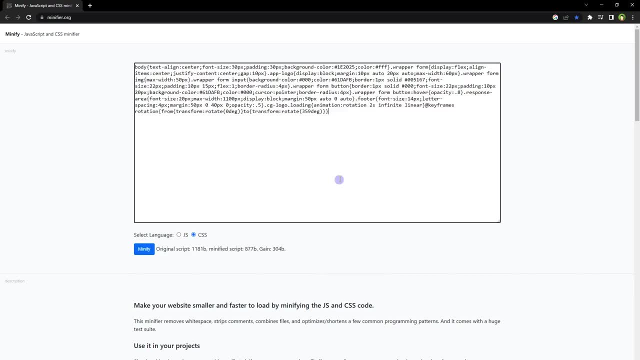 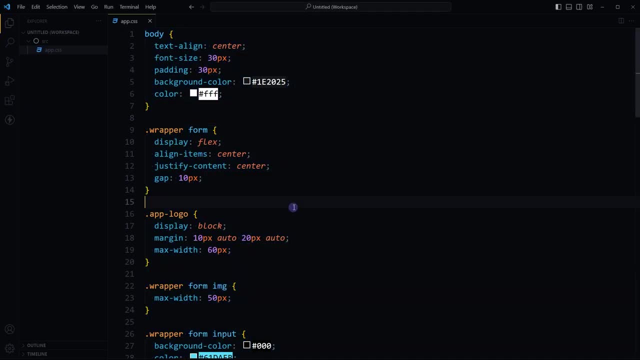 file. Click minify and it will provide minified CSS code. Code editors can also minify code If you use visual studio code. open directory containing CSS file in visual studio code. It is important don't just open CSS file. open project that has CSS file in it. 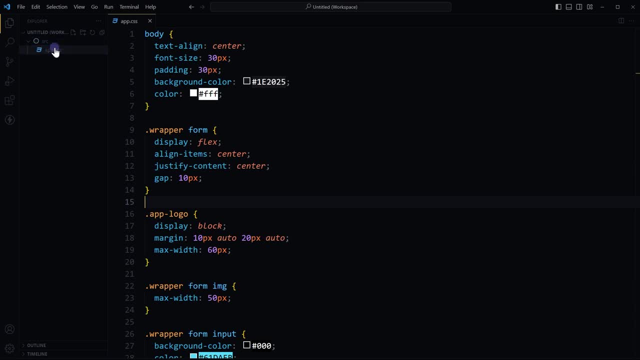 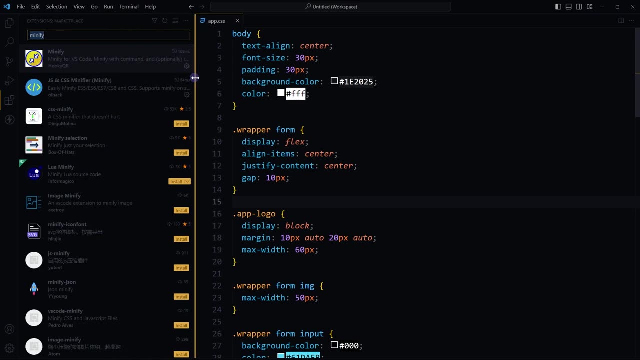 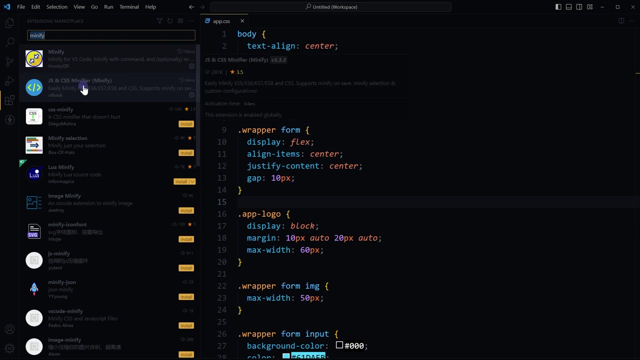 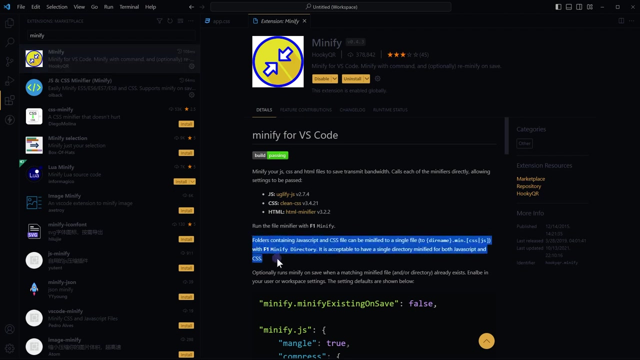 Like. I have opened this project that has got CSS file in it. Search for minify extensions. From extensions search minify. Install any extension related to minification. I have got minify installed. JS and CSS minifier is installed. After installation: enable the extension. Read the instructions about how to use it. 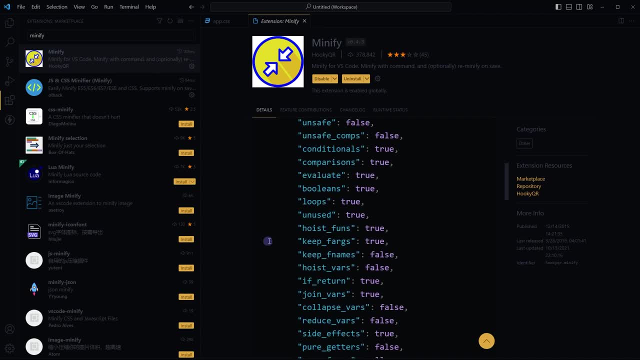 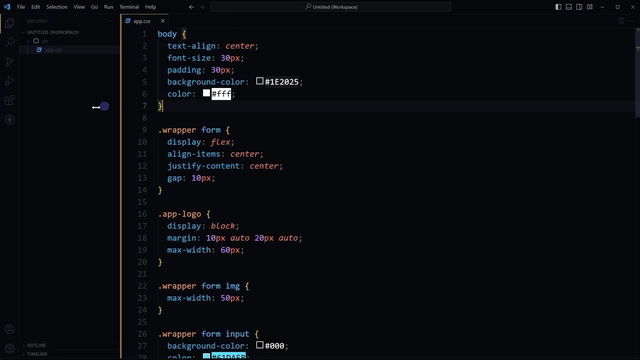 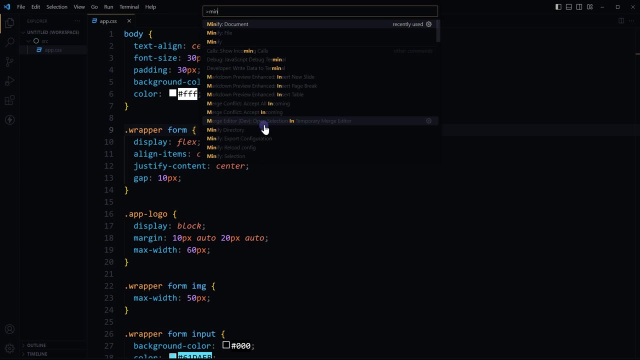 You can also check the settings for the extension that you have installed, But in most cases is that's it. after that open css file, press f1 type minify. you shall see commands related to minification like minify document, minifier file, minified directory. select command that says: 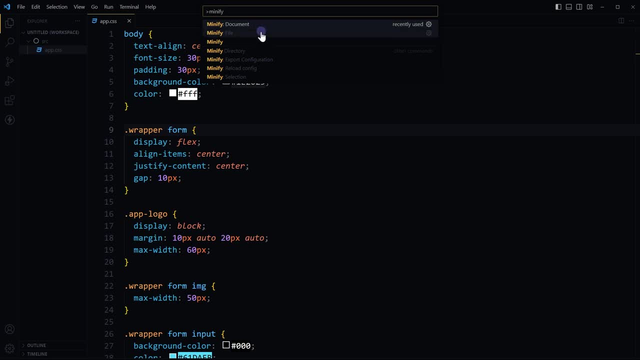 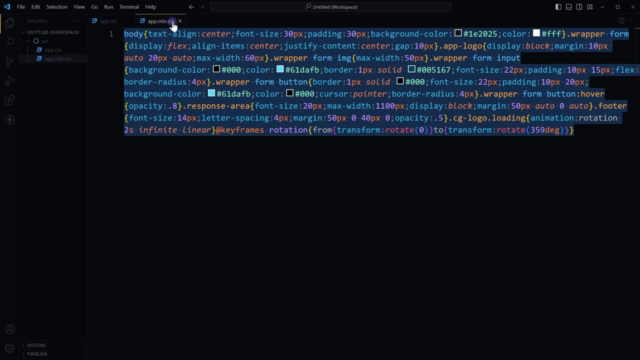 minify file or minified document. select the file that you want to minify and css will be minified in separate file. this is the minifier code in separate file with dot, min. dot. css extension. during the css minification process, various characters such as spaces, tabs, line breaks. 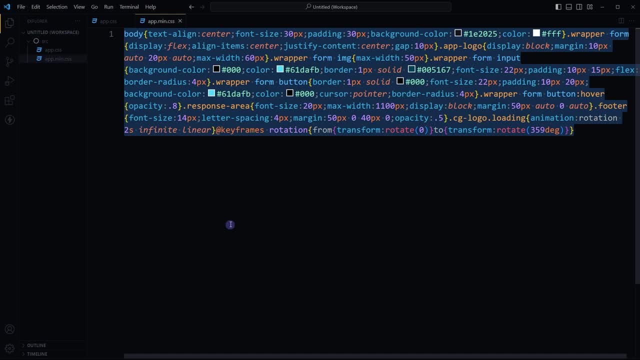 and comments are removed or shortened. however, the css code itself is not altered in any way, so the visual appearance of the web page remains the same. minified css is still valid and can be injured, interpreted by the web browsers and other applications just like regular css it is.